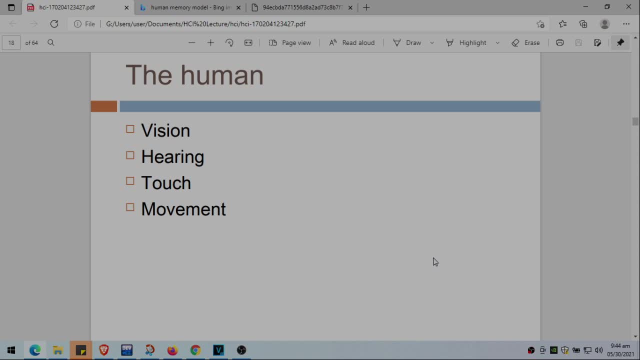 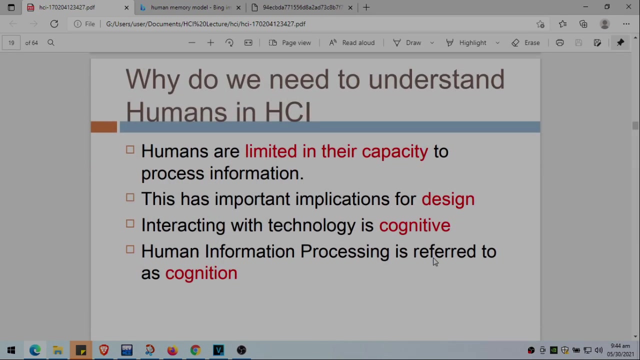 So we can gather information through our vision, through hearing, touch and movement, And this will be discussed in some of our videos on- maybe on our next series- But this is just a short introduction to human Now. why do we need to understand humans in HCI? 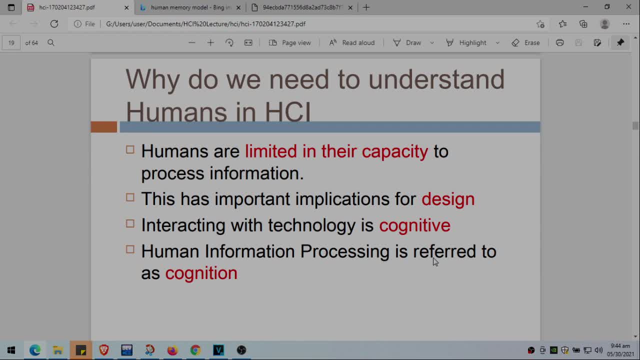 Humans are limited in their capacity to process information And this limitation has an important implications for design Because, again, we don't know the limitations of human, Then maybe our design will not be appreciated by human. Interacting with technology is cognitive. Human information processing is referred to as cognition. 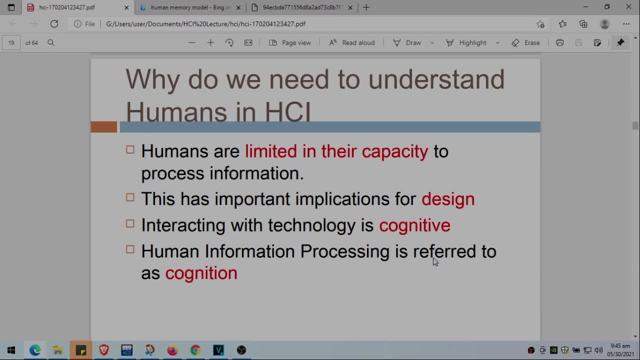 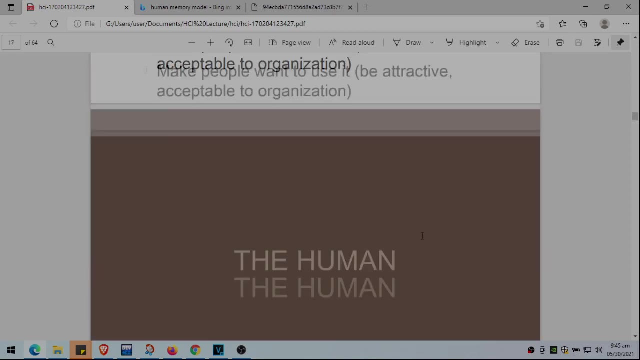 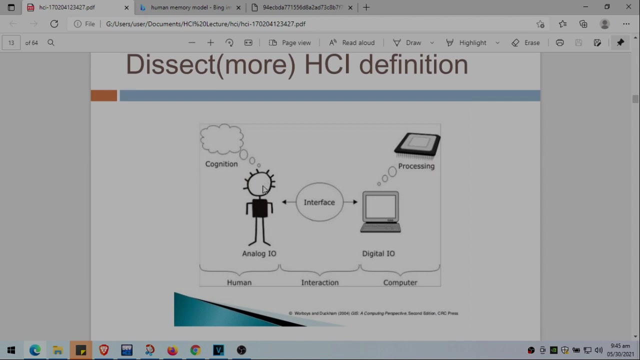 So If a human sees, for example, the user interface of computer, then the human will process this through its cognition. So let's start to get back on our previous slide, last time So here. So we can see here that this is human and this is the computer. 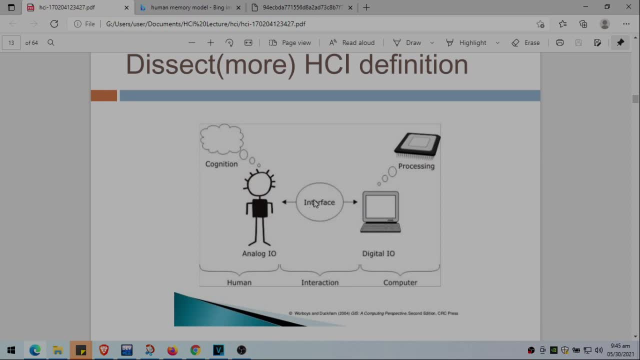 And in between is the user interface or the interface. So the user here, of course, through its vision, maybe we'll see the user interface of the computer, and the human now will of course process that using its cognition. And when it processes that, then the human now will interact or will react with that. 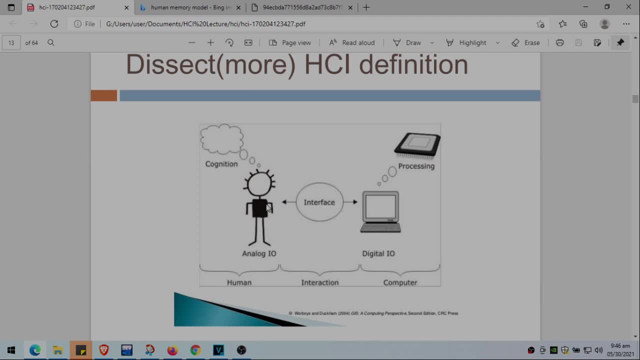 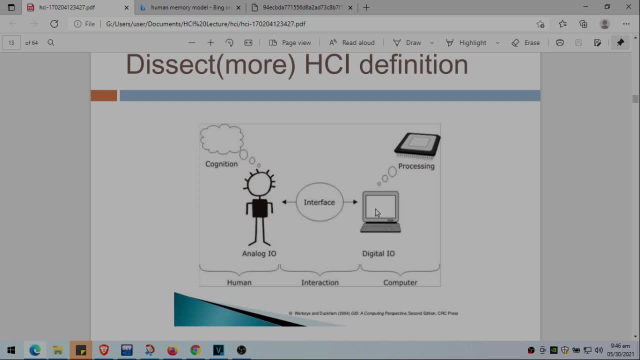 cell phone. So I'll just give an example to make it clearer. Let's say, for example, in the user interface it says here that you have to press the button, or there's a button that will be pressing to submit, for example, the form, so that the 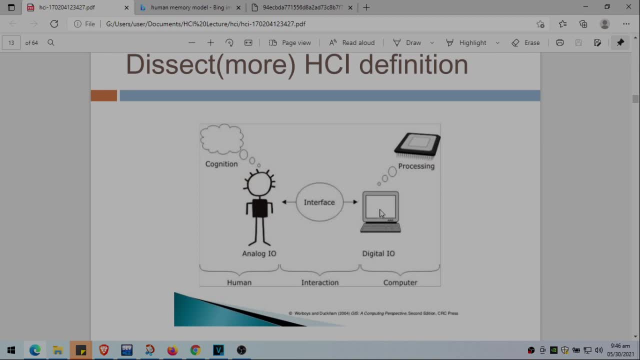 user now could see that form And maybe the user sees the button and that will be processed by the human brain And then, of course, after that is processed by the human brain, the human now will interact with what he sees on the interface. 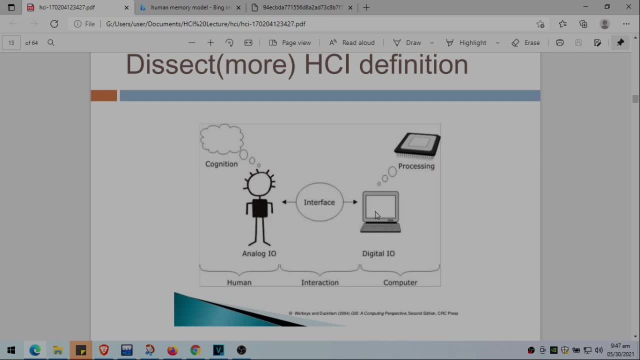 So. so maybe the human now will try to click on the button. so if the button is click, then the computer now will process the action of the human. so that is a human computer interaction. so, as you see here, if the user sees the interface of here, 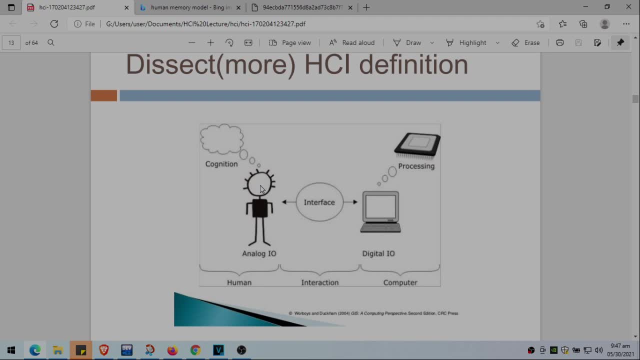 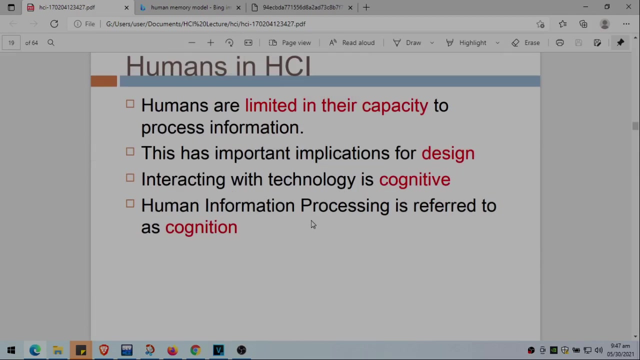 that's why we have here the different inputs for the, or how human gets input like hearing, visual chatter up, so that will be processed by the human and then the human now will interact or where will respond to the stimuli. so let's go back now to our slide. so again human information processing is referred to us. 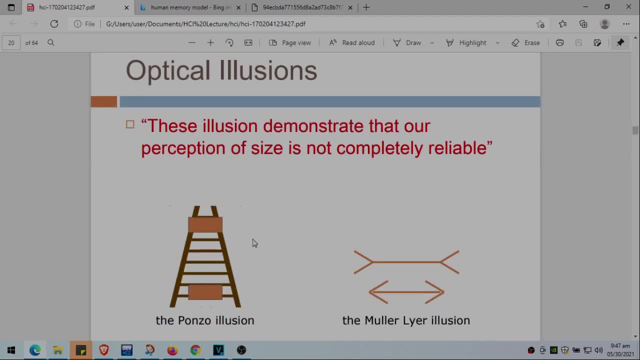 commission. now, here is one of the limitations of human, limitations of human. that's why, again, it's important for us to understand human. so let's say, in this example here we can see that this illusion demonstrate that our perception of sight is not completely reliable. so if you're going to look at this as if this one is bigger than this, but in 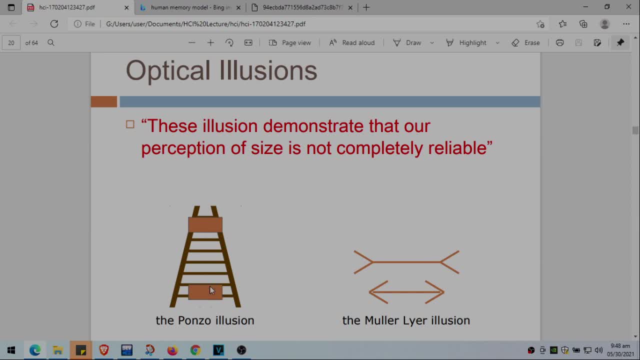 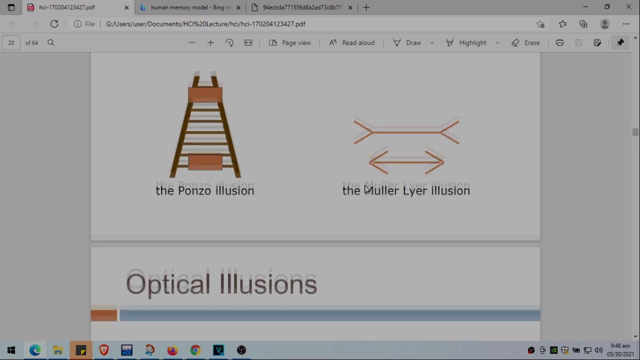 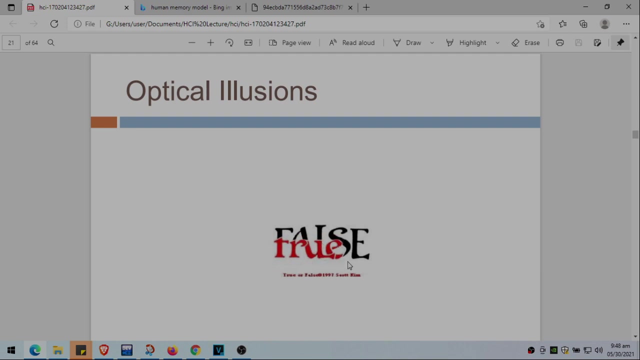 reality they are actually the same size. in this one, the line here seems to be longer than the line here, but in reality- reality- they're also the same, so that means that that is how we, that is, the human perception- is quite unreliable. here's another optical illusion. so we don't know if this is false or true. 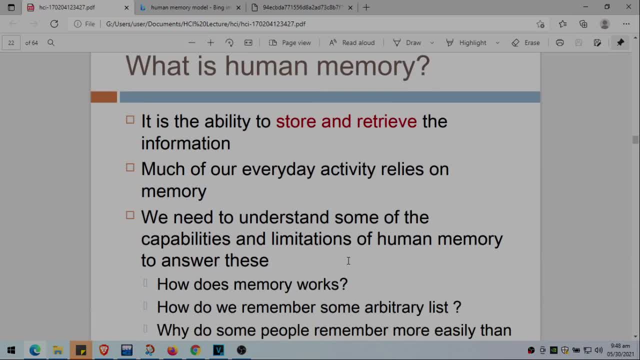 about human memory. human memory memory: it is the ability to store and retrieve the information. much of our everyday activity relies on memory. we need to understand some of the capabilities and limitations of human memory and to answer these: how this memory works. how do we remember some arbitrary is and why? 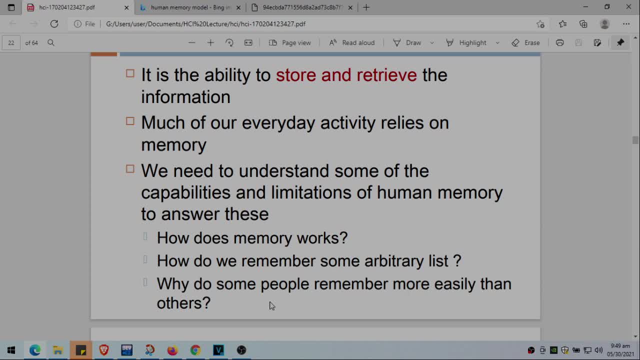 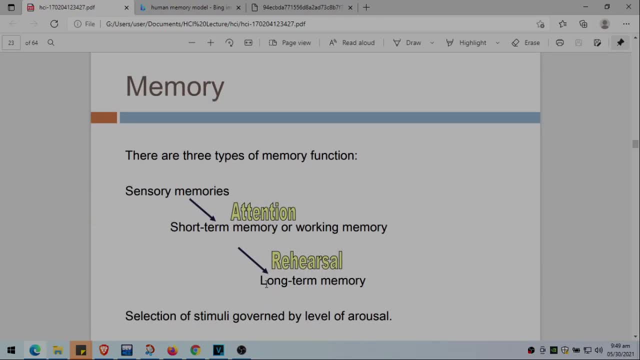 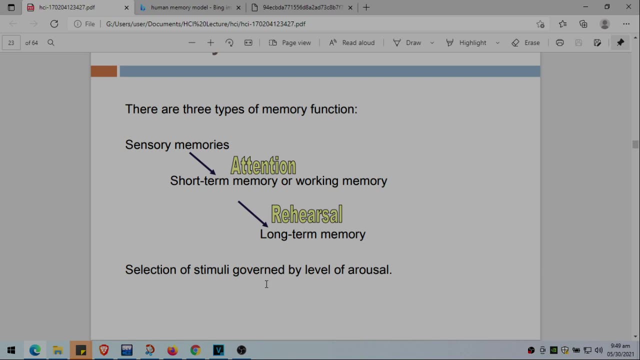 do. some people remember more easily than others- the memory. there are three types of memory function. the first is what we call the sensory memories, or later on I'll be showing you a another diagram. so we have sensory memories and then that will get our attention. and, of course, 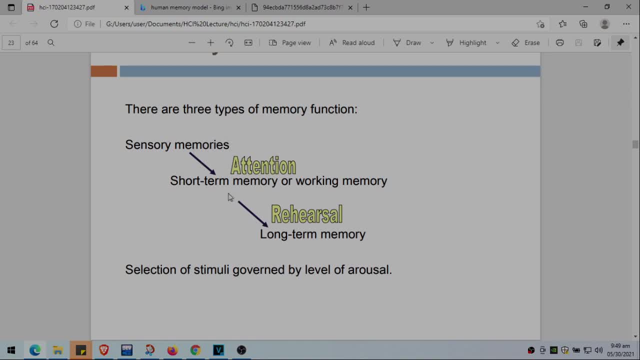 what we see or what we hear will be placed in our short-term memory or working memory, and if this keeps on repeating, then we have what we call some sort of rehearsal and then it will be encoded or placed in our long-term memory. so selection of stimuli governed by level overall. so depends on this then. 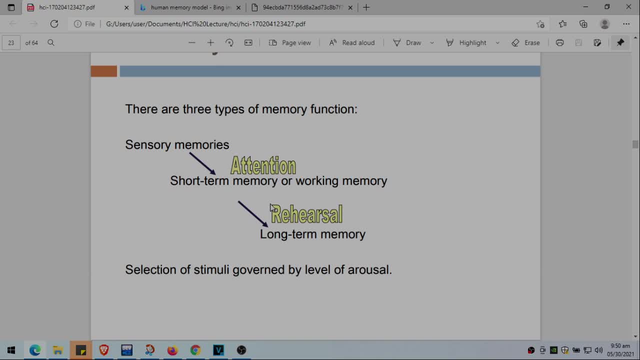 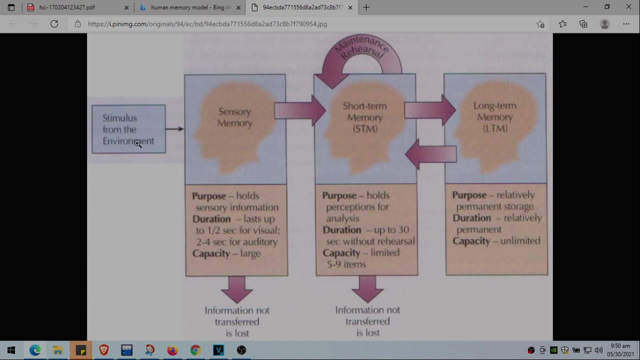 will be reacting to what we see. now let's explain this again taking a look at another chart or image. so here is how it is done. so we see stimulus from the computer, or if it is computed that maybe this is the user interface of the computer, and then that will be of course processed first by our sensory memory. so 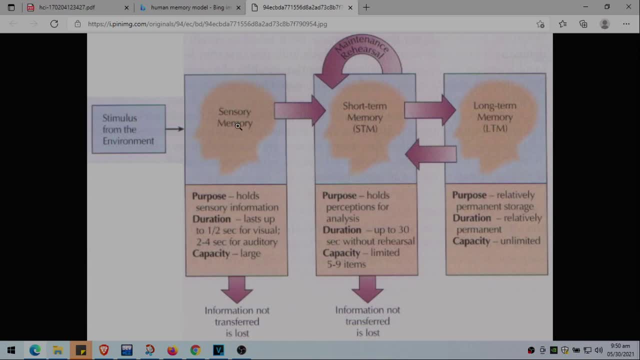 sensory memory has something to do with our senses. so let's say, for example, we see this interface, we could recognize that, oh, this is a button, this is a text box, this one is a menu, so that sensory memory, so the purpose holds sensory memory to the body. so how do we see, how do we see things in light and dimmed? 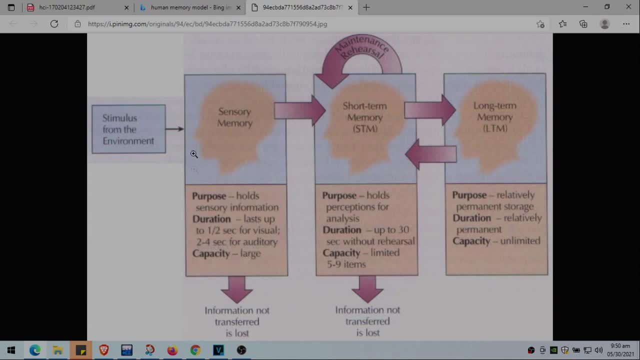 so this is sad, and then we have explained this clearly. so left does not mean you say big or the right, we what we can already see. it may be little bit different, but you can understand it and then set it at that level. upon that, we have the ability to see various things in theseippic visual. 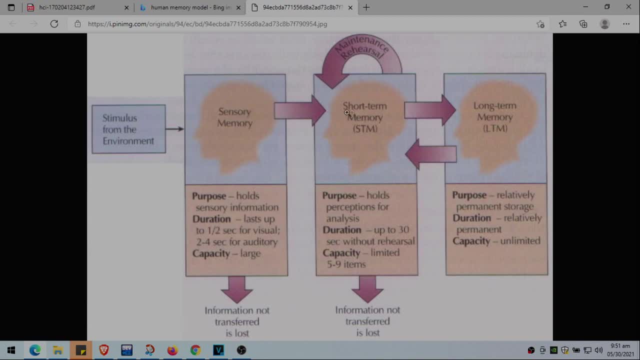 how should we identify these phenomena in our visual Material goes to our short-term memory, so the purpose was again in the short-term memory. the purpose holds perception for analysis. so we'll be trying to analyze what we have seen. so it's a button then maybe we analyze. also we could say to: 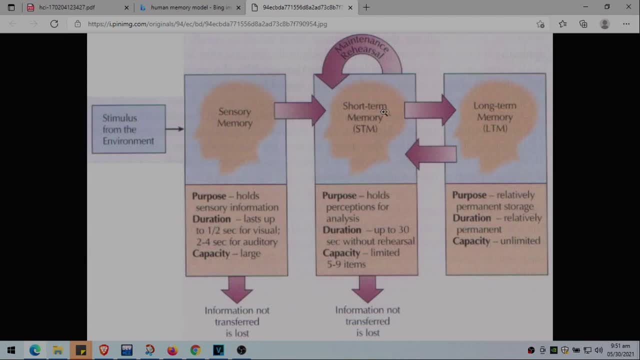 our mind that all this button, we can click on this button to do this, etc. so duration is up to 30 seconds without rehearsal and capacity limited to five to nine items. so with this we can this one also, as the capacity has a implications to design, especially in your user interface. so again, information. 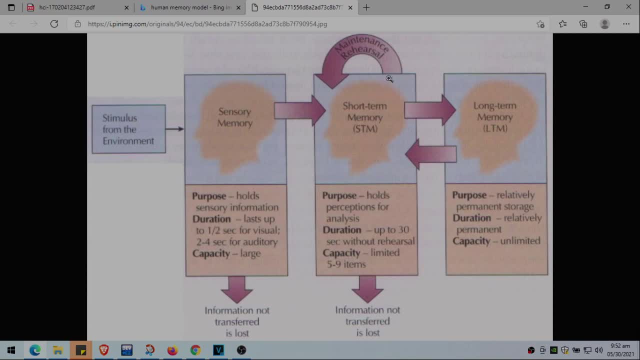 not transferred can be lost. but you can see here that we have to maintenance, rehearsal. so what if we see the same user interface every day? then most probably it will not be, just will not be just placed in our short-term memory, but we place on our long-term memory. so the purpose here is: 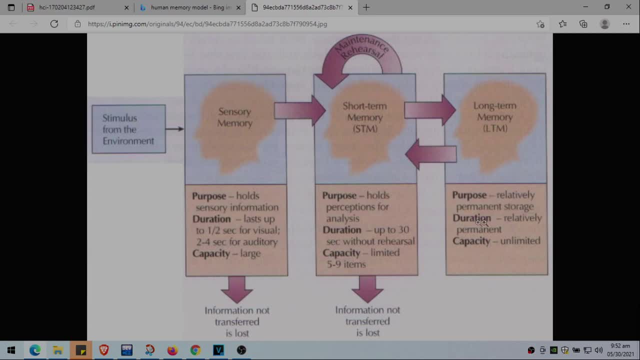 relatively permanent. storage duration is relatively permanent, such even, let's say, after days or even years. sometimes you can still remember the user interface because of it was rehearsed several times in your short-term memory. then the capacity is also unlimited. you see this arrow here. sometimes our short-term 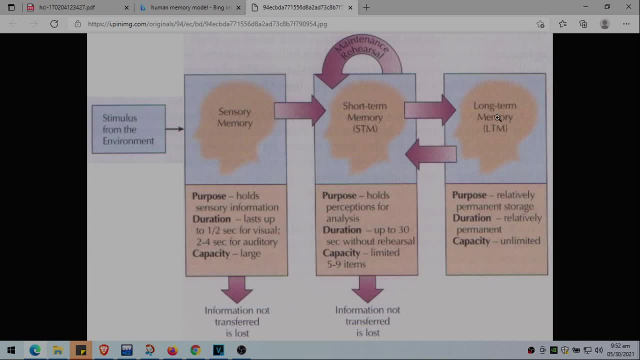 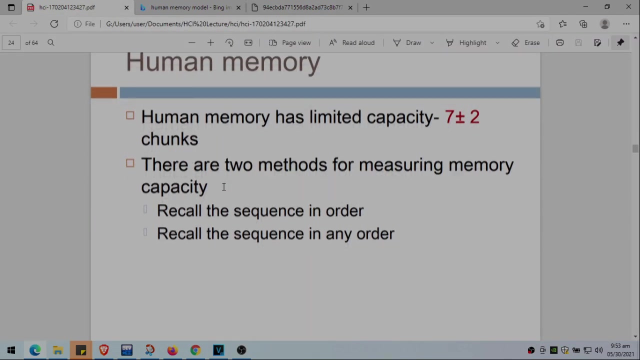 memory. we have to, for example, retrieve it from our long-term memory so that it will be processed, and short-term memory, and this is how our memory works. so the human memory has limited capacity of seven plus or minus two chunks. there are two methods for measuring memory capacity: recall the sequence in order, or 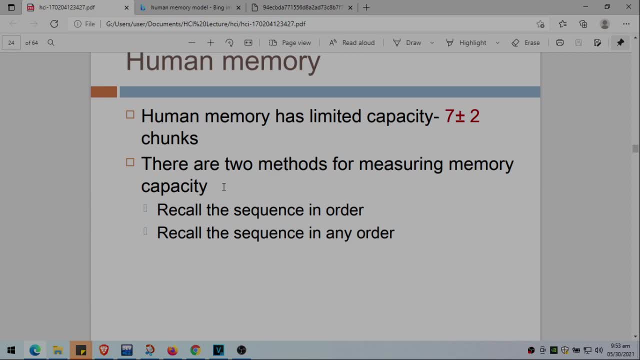 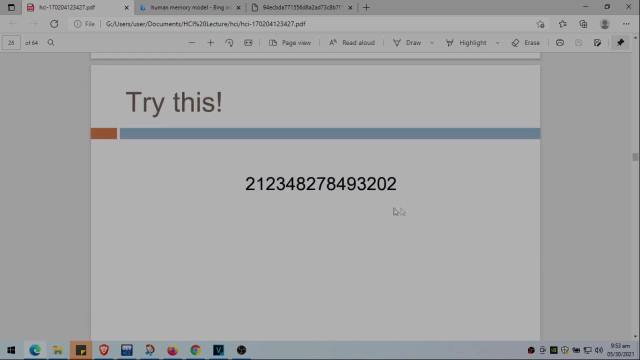 and recall the sequence in order, in any order. so let's try this. for example, could you memorize this number? sometimes it will be very hard to memorize this number, but what do humans do, especially, for example, your cell phone number? what do you do with your? 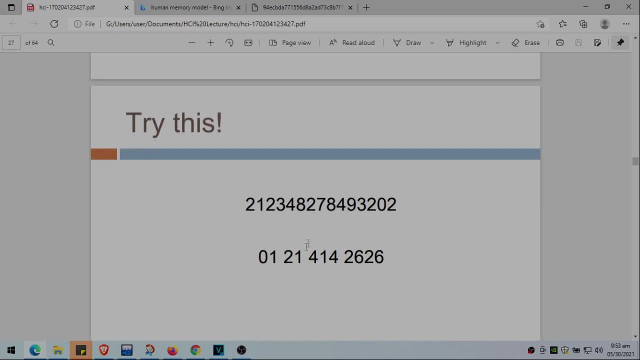 cell phone number. usually what we do is we try to break it into chunks. that's why, for example, if you have your cell phone number, you just you don't memorize the eleven numbers directly, or you don't let's say mention or, yes, memorize your. 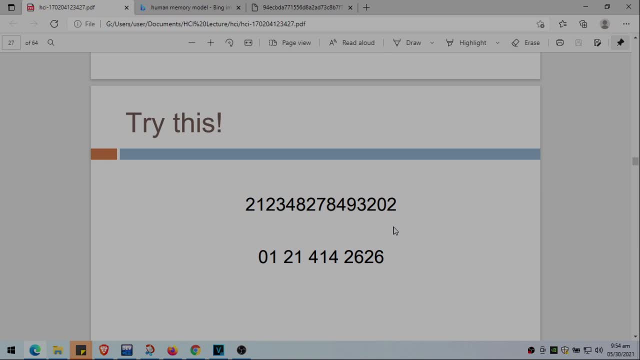 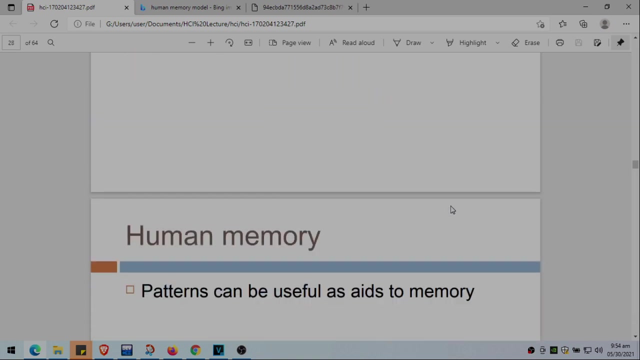 cell phone, cell phone number: the eleven numbers at once, but what you do is to more or less divided into chunks, like, for example, zero, nine, two, seven, five, five, three, four, five, six, four. so we just try to divide into three groups, and that's how we try to memorize things. and 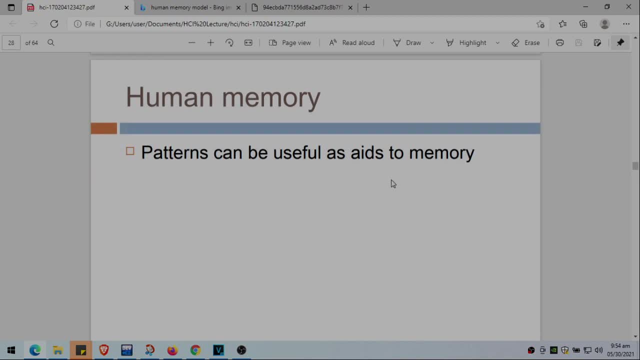 patterns can be useful also as aids to memory. so can you memorize this? you can memorize this and you can memorize this and you can memorize this. you can memorize this and you can memorize this and you can memorize this. you can memorize this and you can memorize this. maybe it will be very difficult. 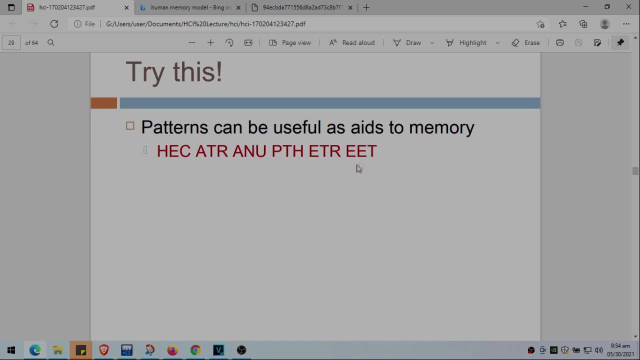 maybe it will be very difficult. maybe it will be very difficult, although this one is already grouped, we, although this one is already grouped, we, although this one is already grouped, we already have chunks, but still it may be already have chunks, but still it may be already have chunks, but still it may be difficult if it is just like this. but 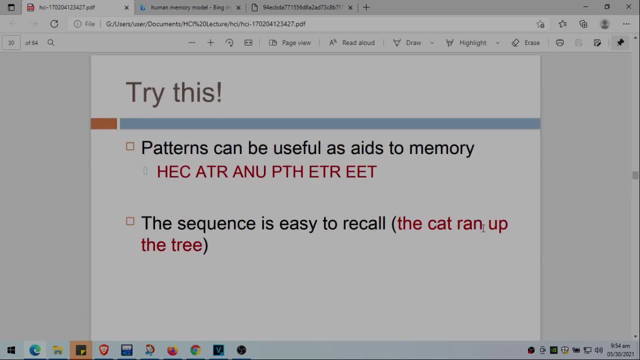 difficult if it is just like this, but difficult if it is just like this. but what if I? what if I? this actually is the. what if I? what if I? this actually is the what if I, what if I? this actually is the same as this, except that the letter T. 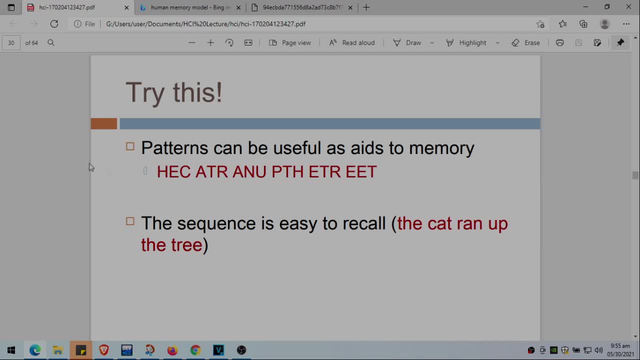 same as this, except that the letter T same as this, except that the letter T here is on the place on the first before. here is on the place on the first before. here is on the place on the first before the first letter. that's right, it became. 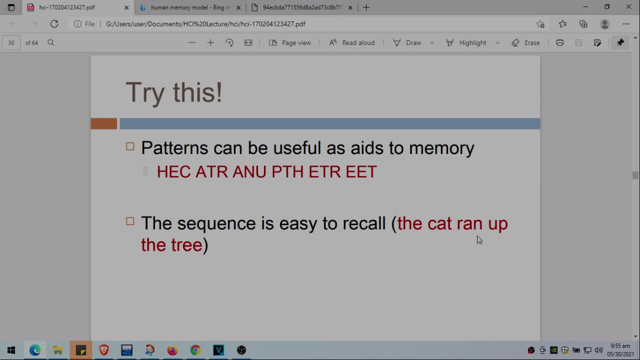 the first letter. that's right. it became the first letter, that's right. it became: the cat run up the tree, so the cat run. the cat run up the tree, so the cat run. the cat run up the tree, so the cat run up the tree will be easier to memorize. 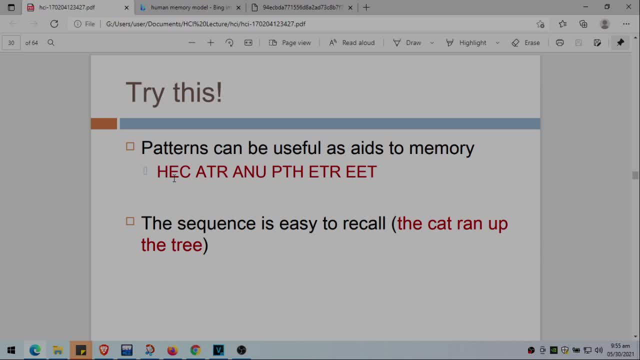 up the tree will be easier to memorize. up the tree will be easier to memorize that HEC 80 are a new PTH 80 are EET. that HEC 80 are a new PTH 80 are EET. that HEC 80 are a new PTH 80 are EET. but if we got to look at this they're. 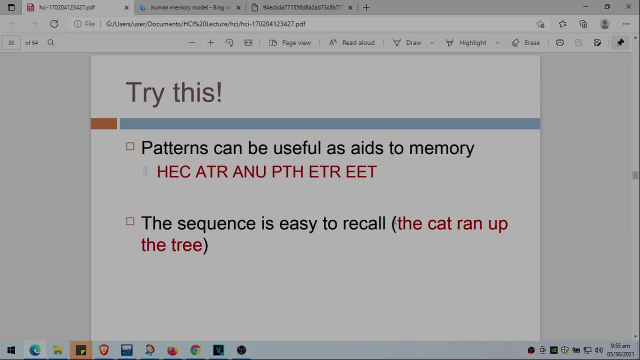 but if we got to look at this, they're, but if we got to look at this, they're actually almost the same, except that the actually almost the same, except that the actually almost the same, except that the letter T here was placed before, the letter T here was placed before the. 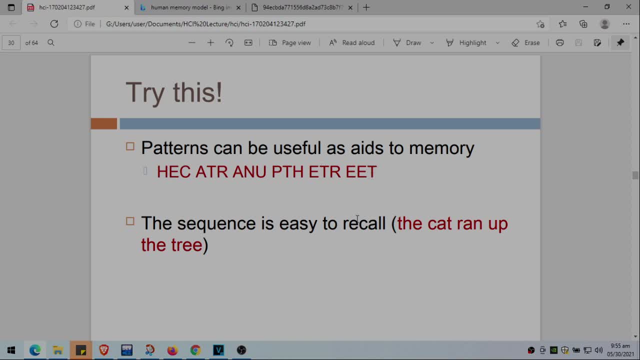 letter T here was placed before the letter H, so the letter T here was placed letter H, so the letter T here was placed before the letter T here. but these are before the letter T here was placed before the letter T here. but these are before the letter T here. but these are the same words, so that's just a teaser. 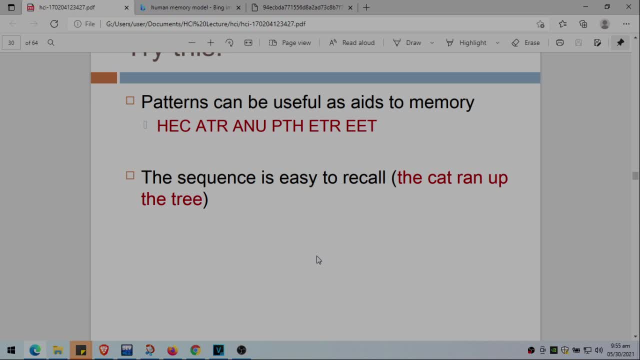 the same words, so that's just a teaser. the same words, so that's just a teaser, of the limitations of human in some of of the limitations of human, in some of of the limitations of human, in some of our next videos we'll be talking about. our next videos we'll be talking about 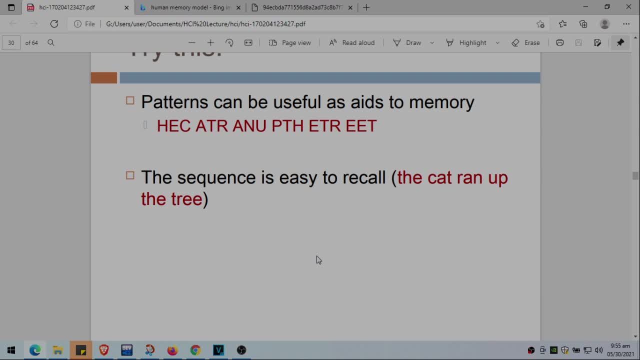 our next videos we'll be talking about human psychology, a human vision, etc. so human psychology, a human vision, etc. so human psychology, a human vision, etc. so for now, we'll be ending this second. for now, we'll be ending this second. for now we'll be ending this second lecture series and thank you very much.